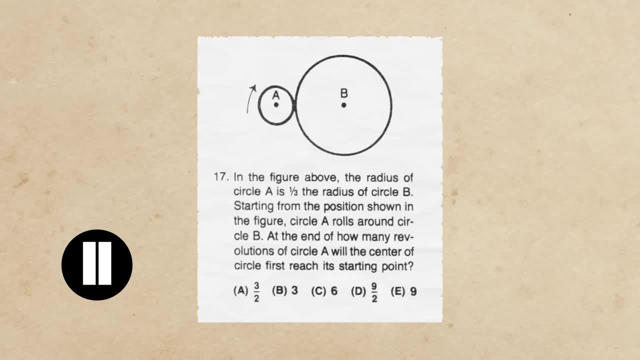 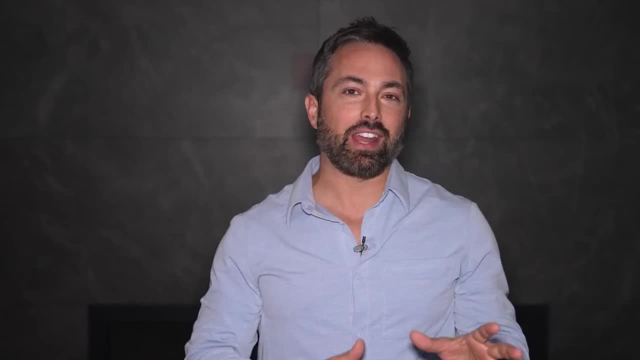 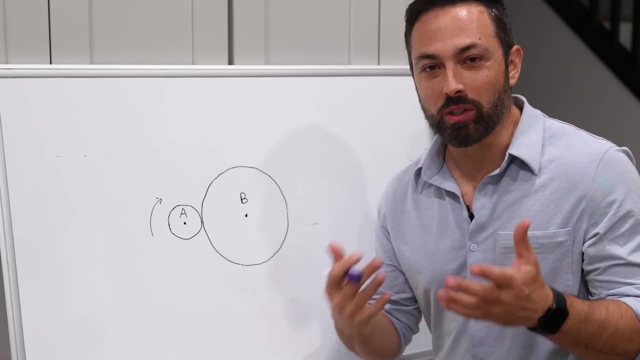 so about a minute each. So feel free to pause the video here and try to solve it. What is your answer? I'll tell you right now that option B or three is not correct. When I first saw this problem, my intuitive answer was B, because the circumference of a circle is. 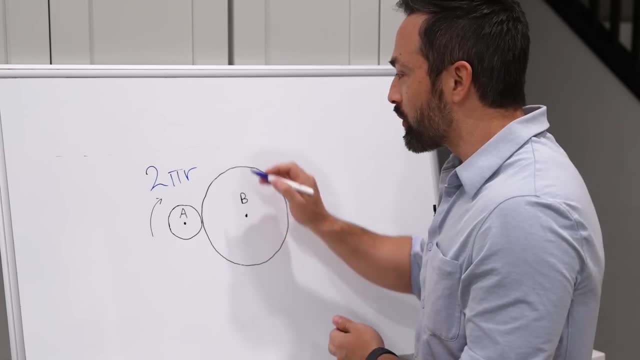 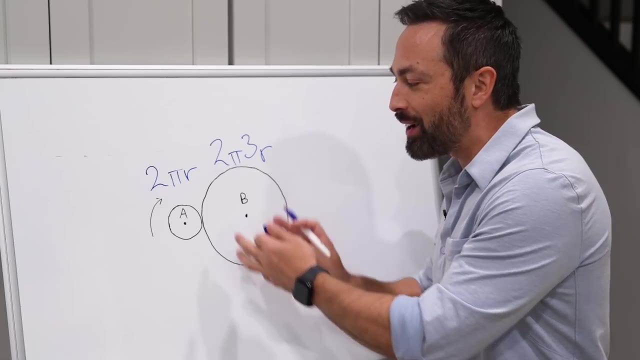 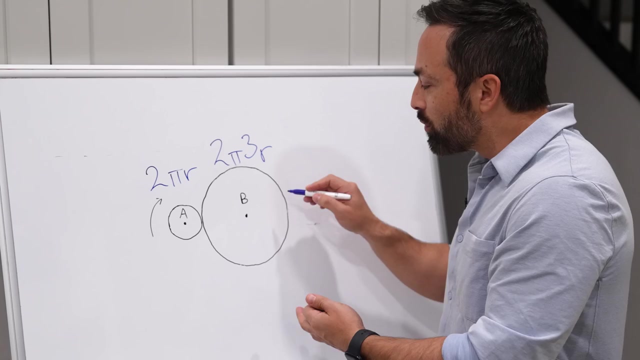 just 2 pi r. and since the radius of circle B is three times the radius of circle A, the circumference of circle B must also be three times the circumference of circle A. So logically, it should take three full rotations of circle A to roll around circle B. So my answer: 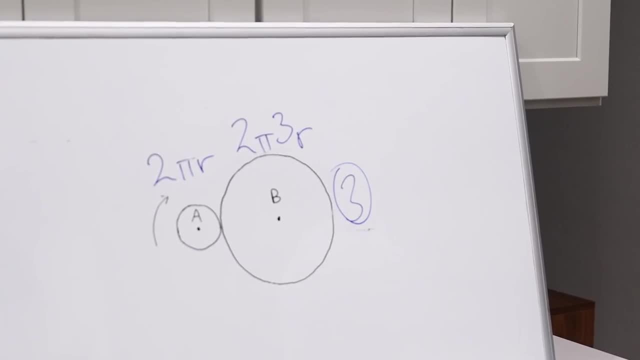 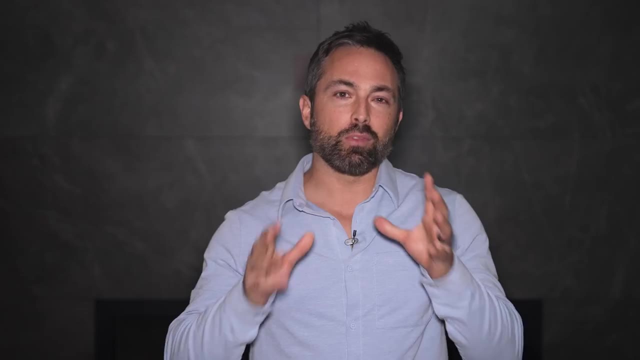 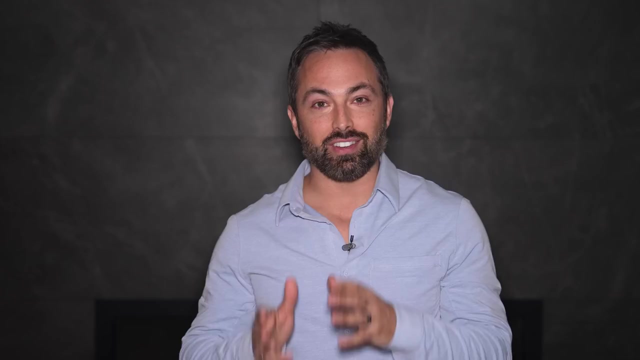 was three. This is wrong, But so are answers A, C, D and E. The reason no one got Question 17 correct is that the test writers themselves got it wrong. They also thought the answer was three. so the actual correct answer was not listed as. 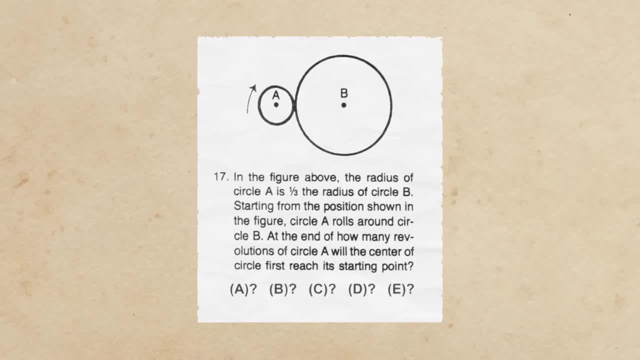 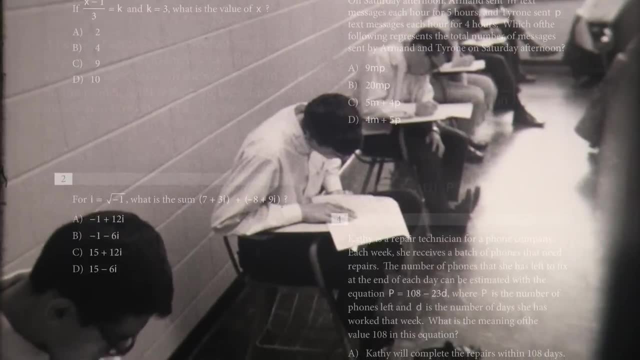 an option on the test. Mistakes like this aren't supposed to happen on the SAT. For decades it was. It was the one exam every student had to take to go to college in the US. It had a reputation for determining people's entire futures. 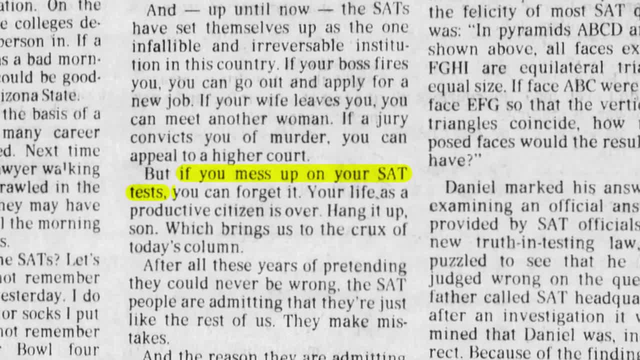 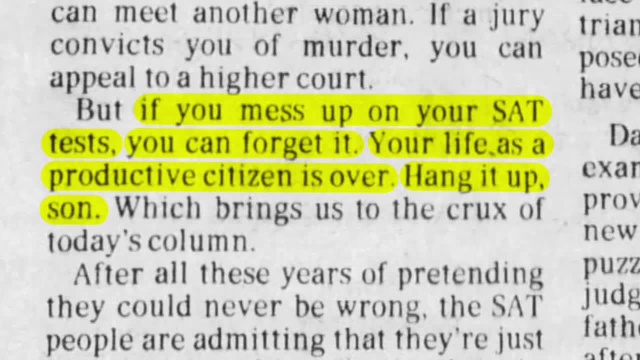 As a newspaper from the time stated, if you mess up on your SAT tests, you can forget it. Your life as a productive citizen is over. Hang it up, son. Of 300,000 test takers, just three students wrote about the error to the College Board. 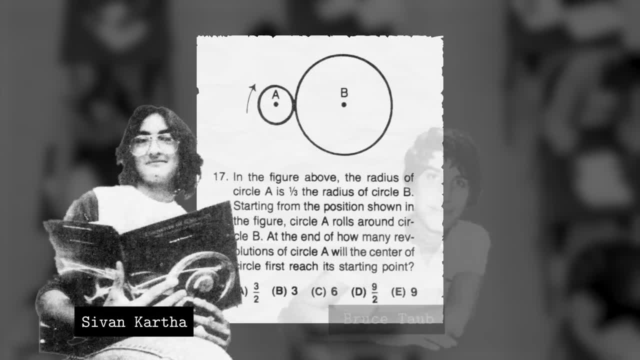 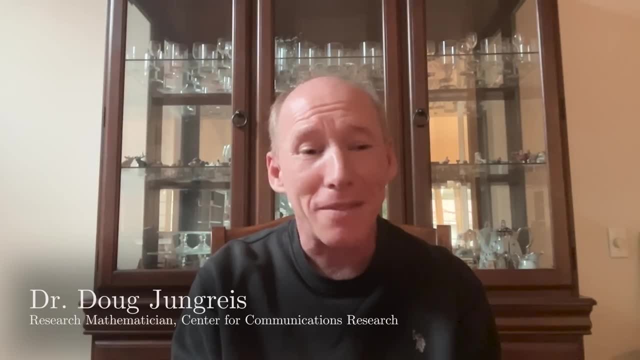 the company that administers the SAT: Shivin Kartha, Bruce Taub and Doug Youngrice. I did a lot of math problems when I was young. For the competitions I probably did thousands of math problems. I read it and I was amazed how badly it's worded. 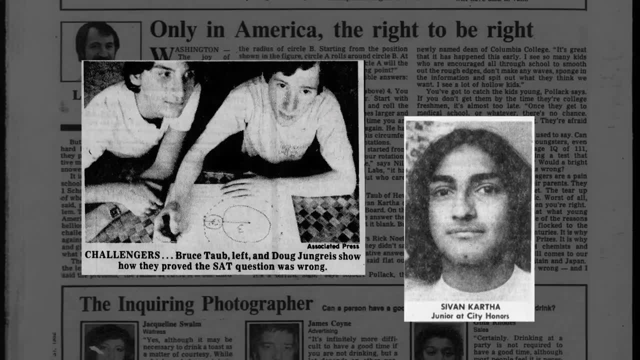 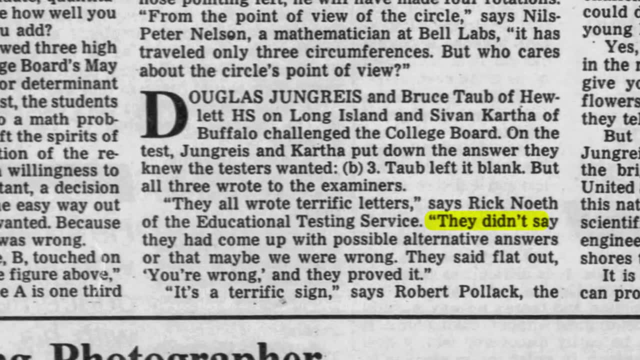 I just put three down. I figured that's what they wanted. The three students were confident none of the listed answers were correct and their letters showed it. As a director at the testing service recalled, they didn't say they had come up with possible. 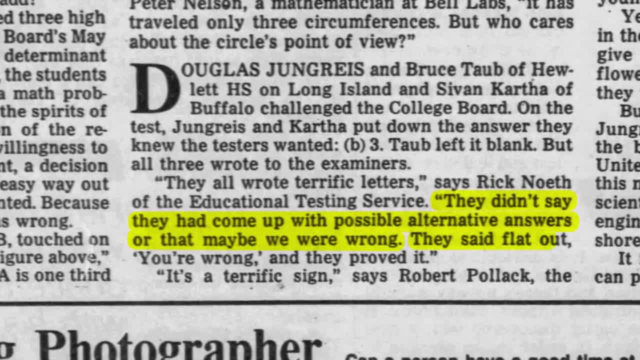 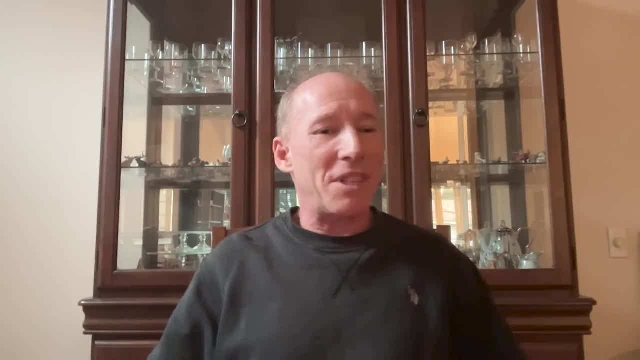 alternative answers or that maybe we were wrong. They said flat out: you're wrong and they proved it. I discussed it with some other people and said I think there was a mistake and they mostly said no one cares. I wrote a letter to the educational testing service. 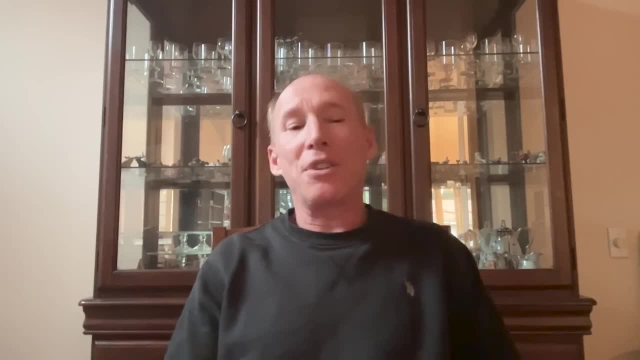 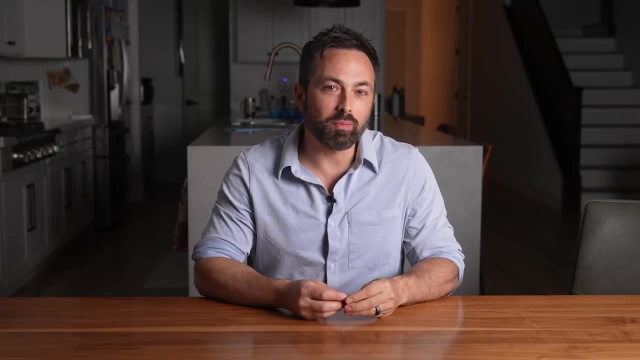 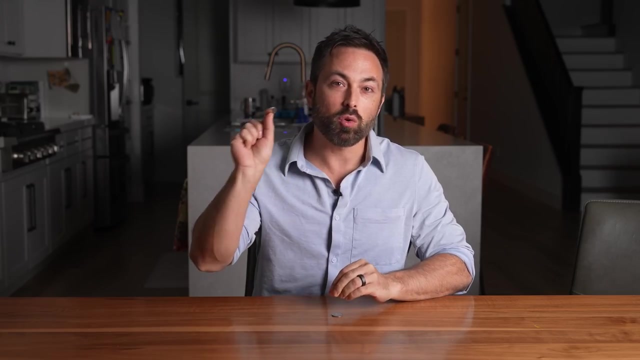 It was a little while later They called us and said I was correct. Here is their argument. The simplest version of this problem is with two identical coins. These have the exact same circumference, So by our initial logic, this coin should rotate exactly once as it rolls around the 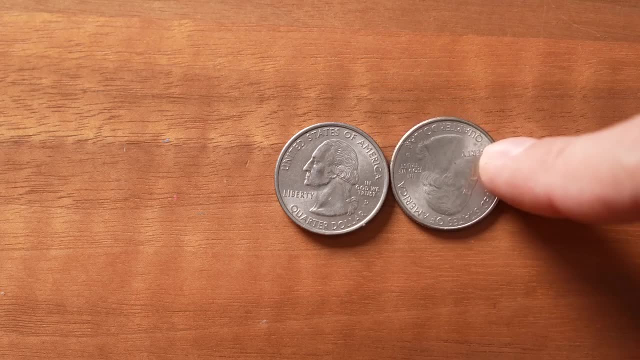 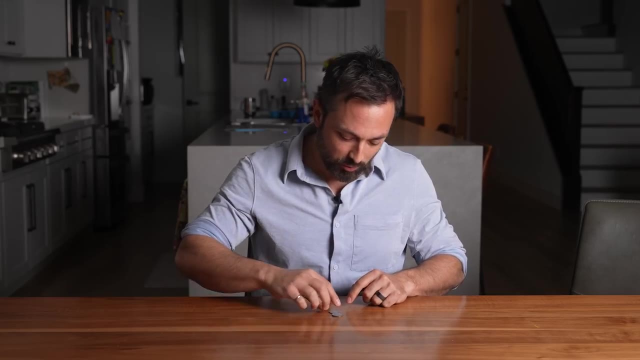 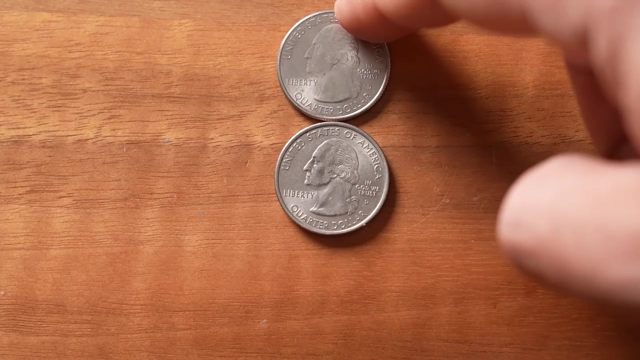 other. So let's try it. But wait, we can see it's already right side up at the halfway point. So if we finish rolling it around the other coin, it'll have rotated not once but twice, Even though the coins are the exact same size. there are no tricks here. 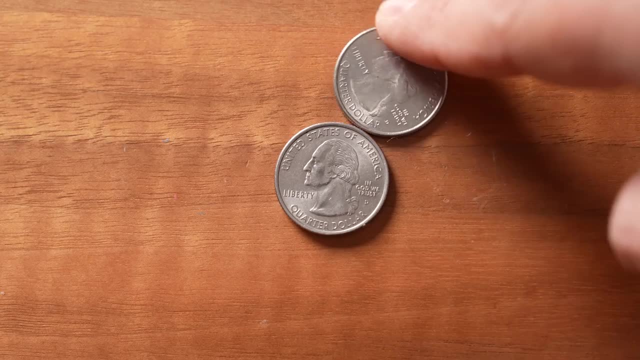 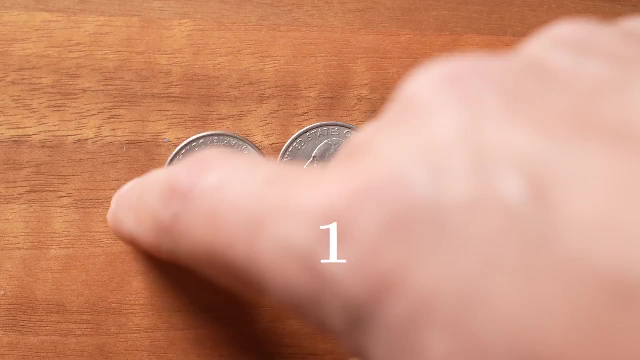 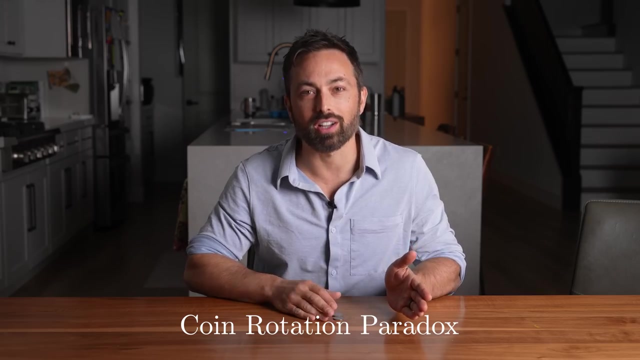 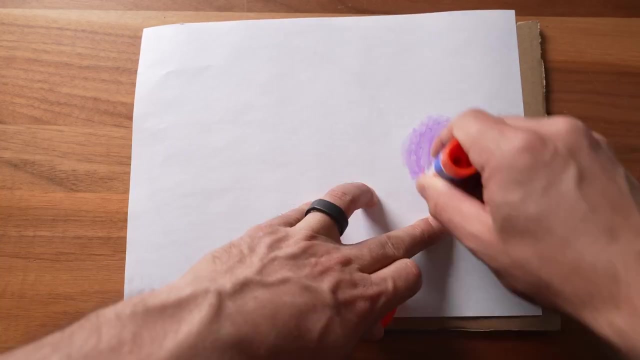 You can try it for yourself and I'll do it again slowly. So one, two. So this is known as the coin rotation paradox. This paradox also applies to question 17.. I've made a two scale model of the problem. One useful tip for standardized tests. 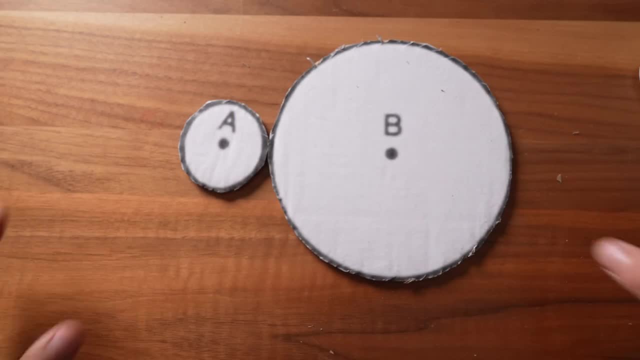 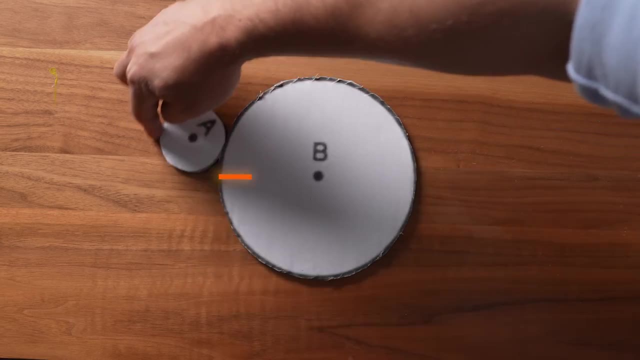 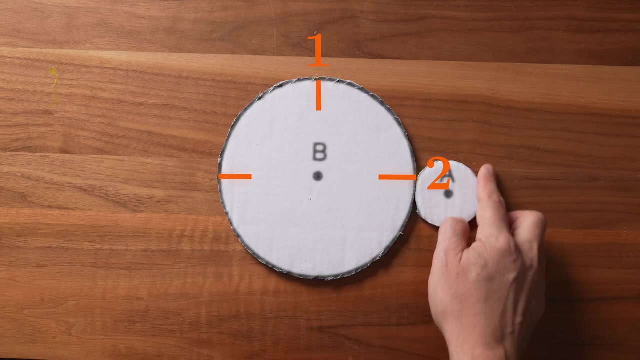 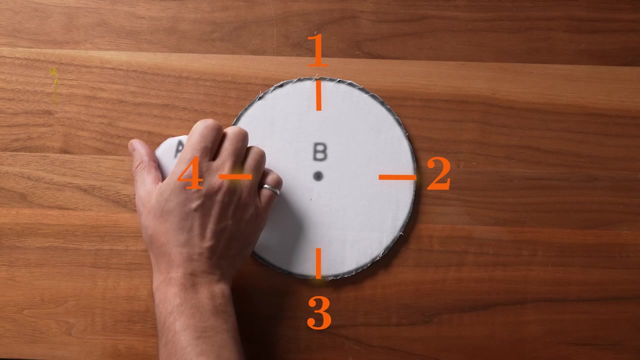 Let's go to question 17.. Question 17.. Second question: scale. they almost always are. So when we roll circle A around circle B, we can see that it rotates once, twice, three times and four times in total. So the correct answer to this question. 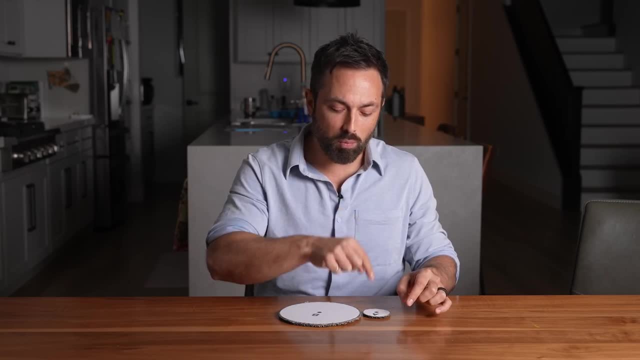 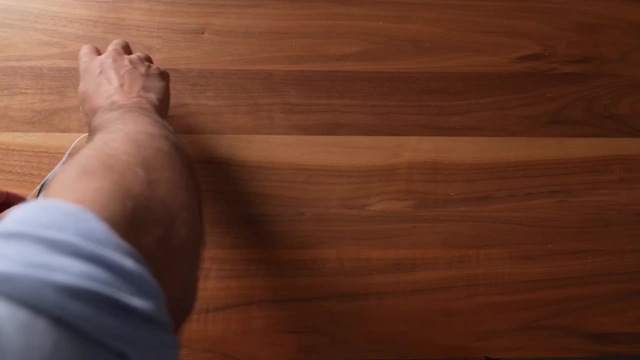 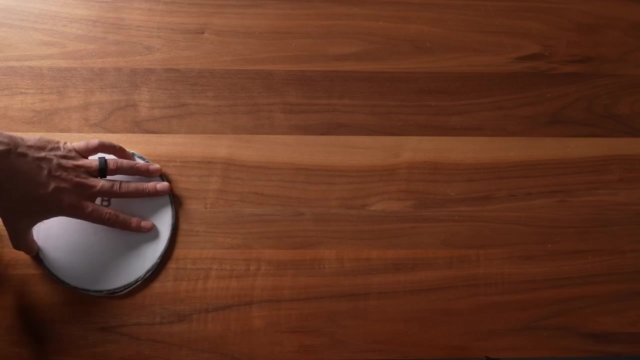 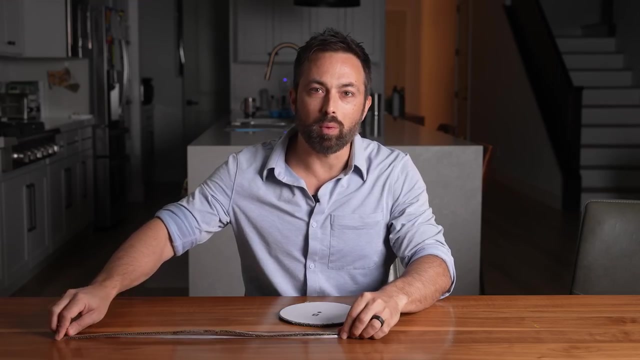 is actually four. Once again, the circle rotates one more time than we expected. To understand this, let's wrap this larger circle in some ribbon And I'll make it the same length as the circumference, And then I will stick it down to the table as a straight line. I'm adding some paper here, So there's something for this to roll. 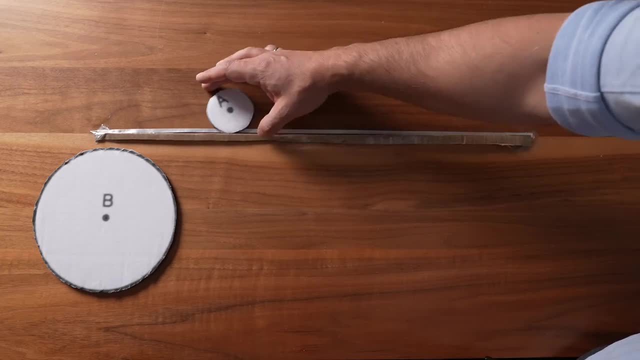 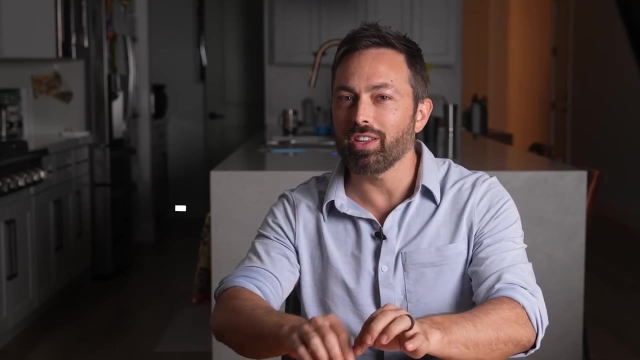 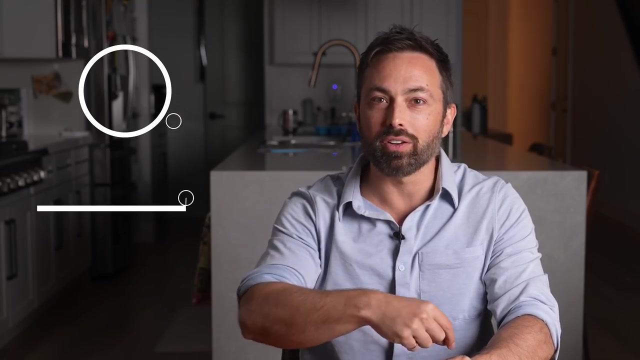 on And now it rolls one, two, three times. What's happening when we turn this straight path into a circular one is that circle A is now rolling the length of the circumference and it's going around a circle. The shape of the circular path itself makes circle A do an additional rotation. 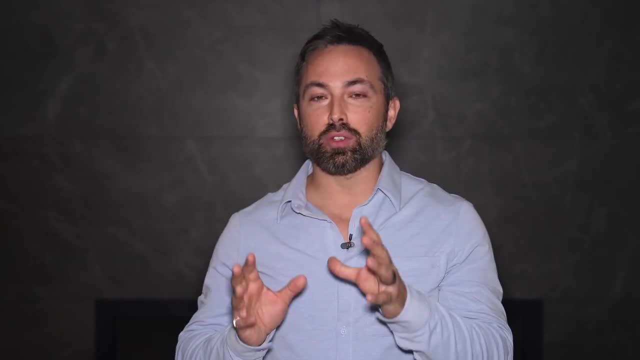 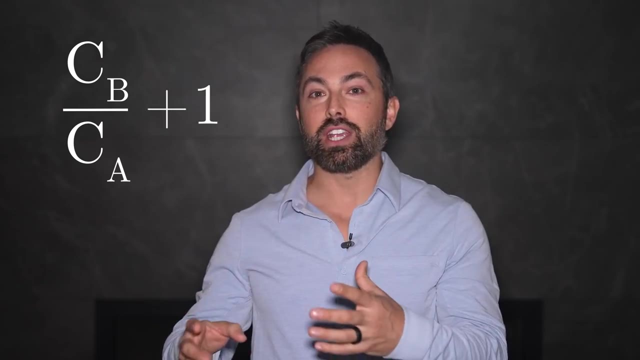 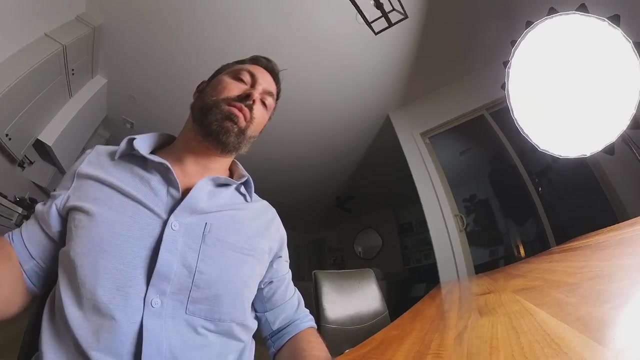 to return to its starting point. So this is the general solution to the problem: Find the ratio between the circumferences of circle B and circle A And then add one rotation to account for the circular path traveled. But there is a way to correctly get three. Let's count the rotations of circle A from: 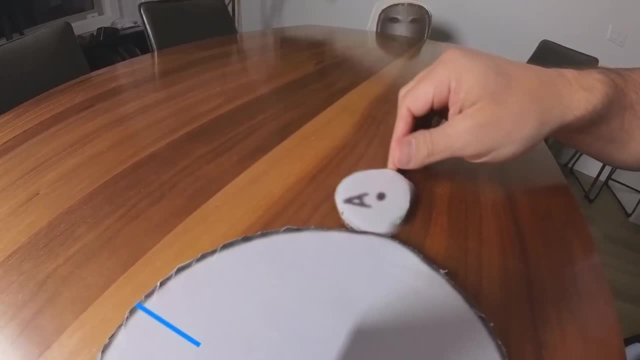 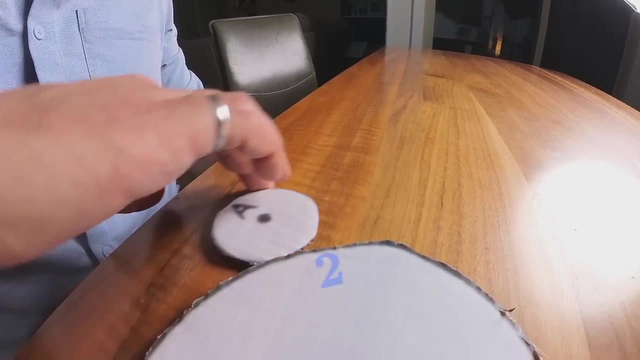 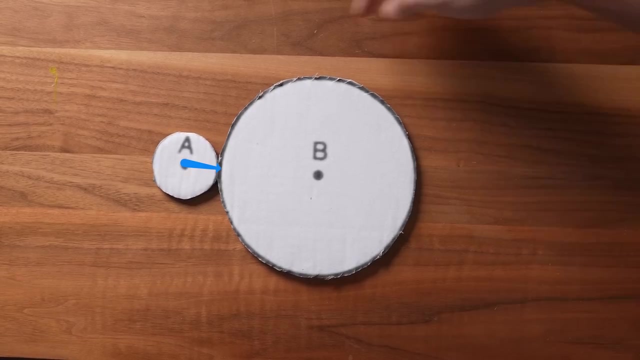 the perspective of circle B. looking out at A, We can see circle A rotates one, two, three times And it doesn't matter which circle you're looking at, It's going to be one, two, three times For each of these three rotations. it rotates up three times as you are looking from there. 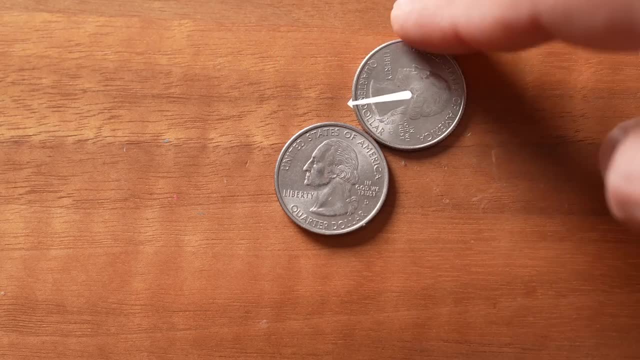 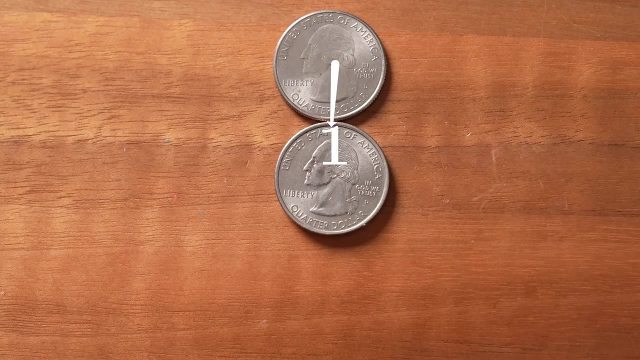 To circle A. it also rotates three times to come back to its starting position around circle B. Similarly, from the perspective of the coin, we can see that the outer coin only rotates once as it rolls around the inner coin. Using the perspective of a circle is just like turning the circle's circumference into a straight line. 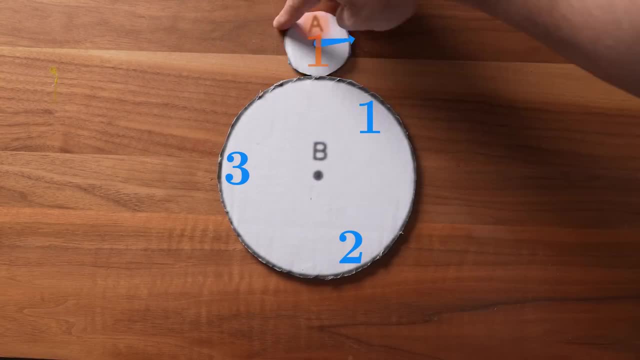 It's only as external observers that we actually see the outer circle travel a circular path back to its starting point. Can you imagine ع Fab K Gr R, greater, equal, higher or different? A book I found online the next day told me the 2nd limit of square Нüzел's contemporaries is xn. Is it right to put xn as the initial value that one points over a circle? varsawn as gives the center value. 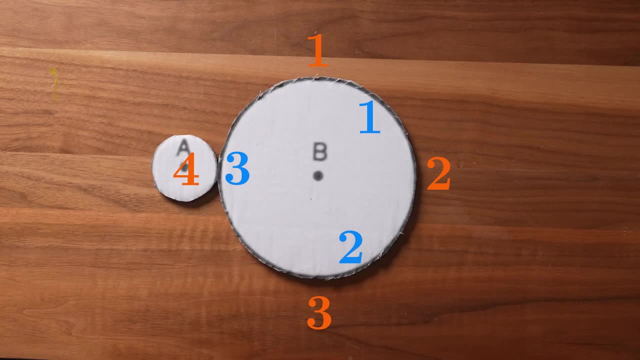 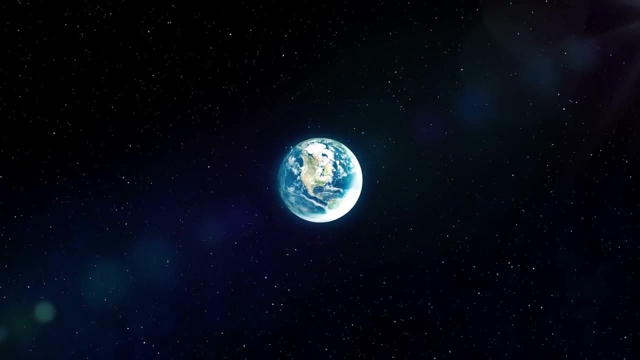 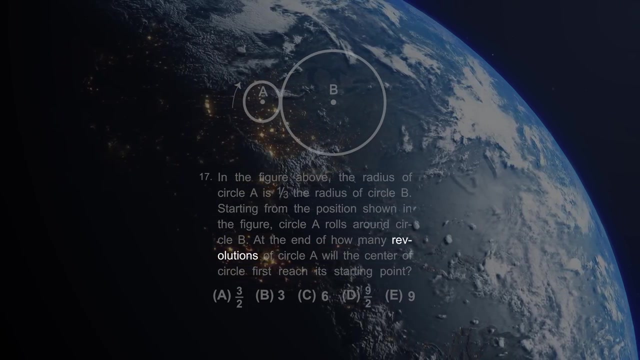 point, giving us the one extra rotation. But there's even another answer, If you look closely at question 17,. it asks how many revolutions Circle A makes as it rolls around Circle B back to its starting point. Now, in astronomy the definition of a revolution is precise. 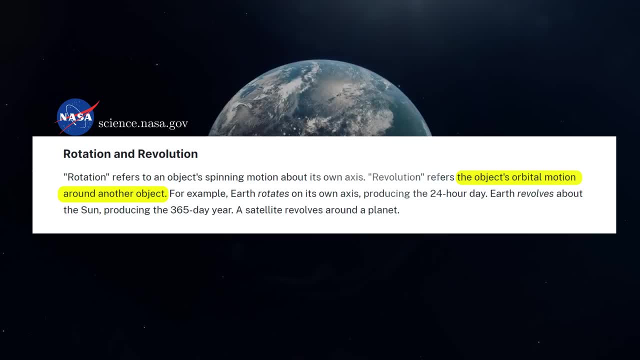 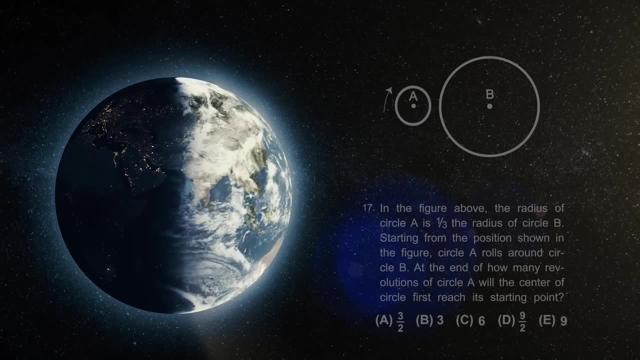 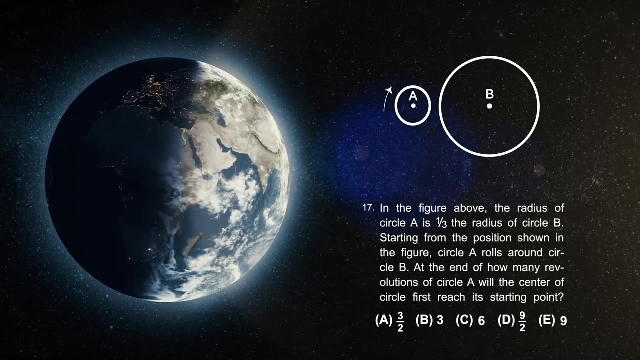 It's a complete orbit around another body. The Earth revolves around the Sun, which is different from it, rotating about its axis. So by the astronomical definition of a revolution, Circle A only revolves around Circle B once It goes around one time. Now, other definitions of a revolution do include the motion of an object rotating about its. 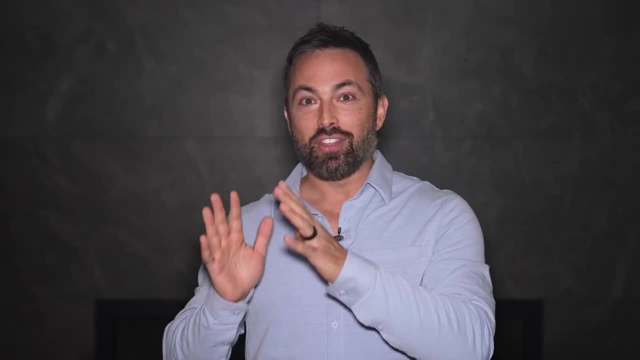 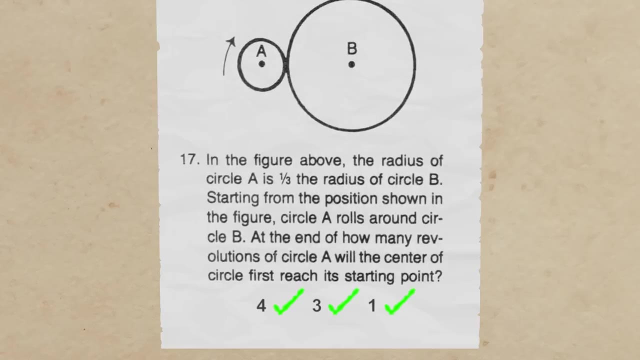 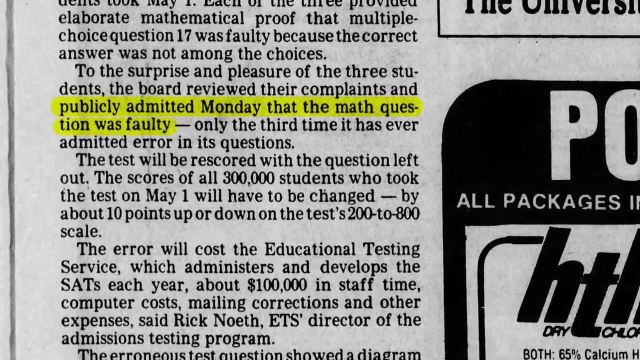 own axis. So one isn't a definitive answer, But the wording of this question is extremely ambiguous. if you can justify at least three different solutions. After reviewing the letters from the students, the College Board publicly admitted their mistake a few weeks later and nullified the question for all test takers. 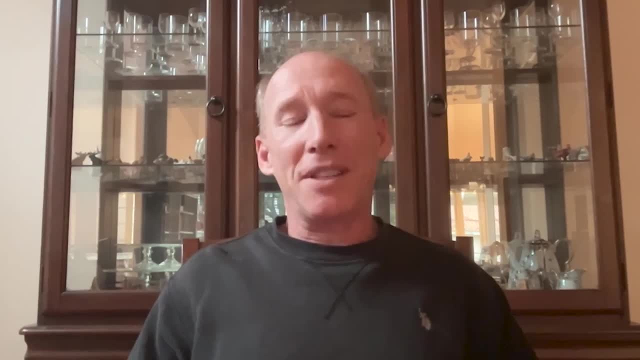 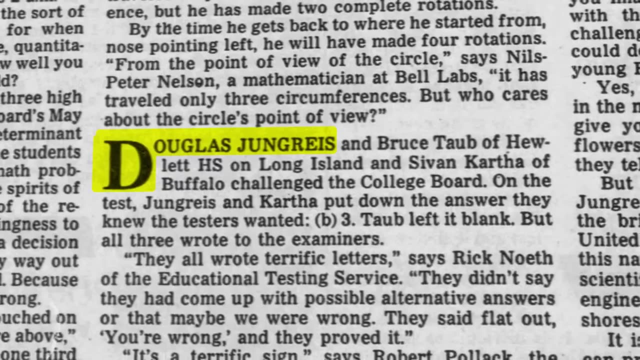 They said they were discounting the problem and they were calling us because they were going to tell the news and they thought that we should be warned that the news might contact us. I did a bunch of phone interviews and NBC News. They came to my school. 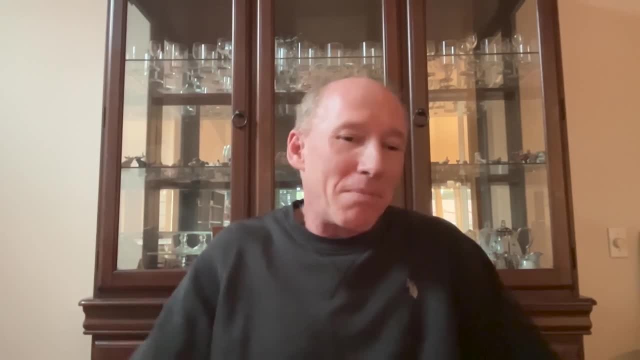 They said they were. they said I was right and they were discounting it. So that was great. But there's more to the explanation. It's easy to get an intuitive reason, but it's really hard to formally prove that the answer is four. 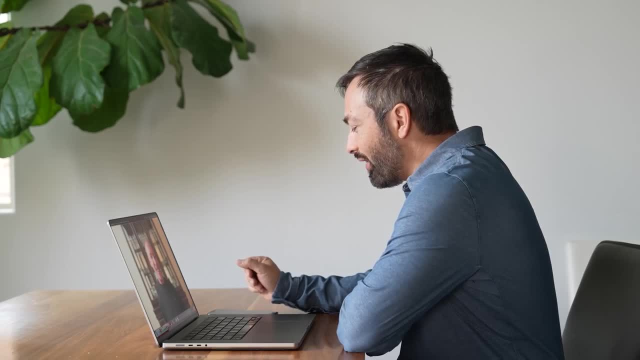 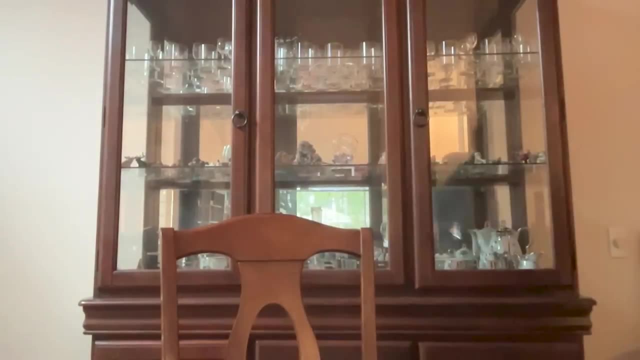 I could give you some proofs if you want. Well, that would be wonderful. I think that would be. we'd appreciate that. for sure, I have a whiteboard because I'm a mathematician, so I just happen to have a whiteboard here. 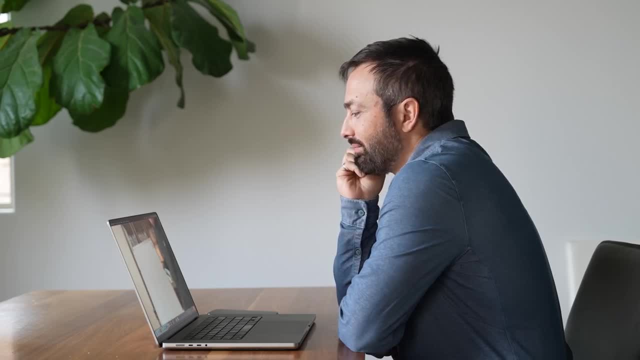 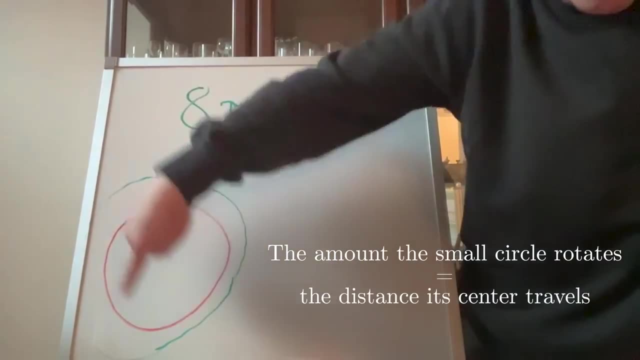 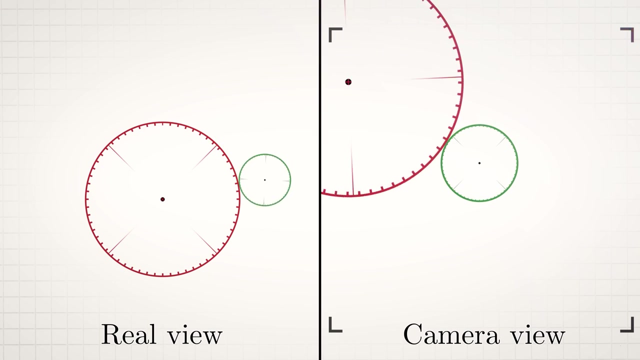 Hold on. Can you see that? Yep, It turns out That the amount That the small circle rotates is always the same as the distance The center travels, All right. So why is this true? Suppose you had a camera, and the camera was always pointed at the center. 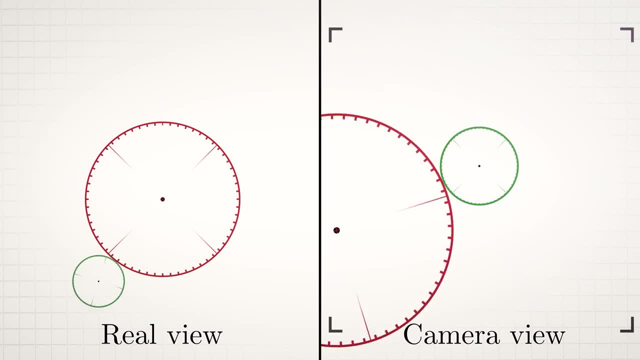 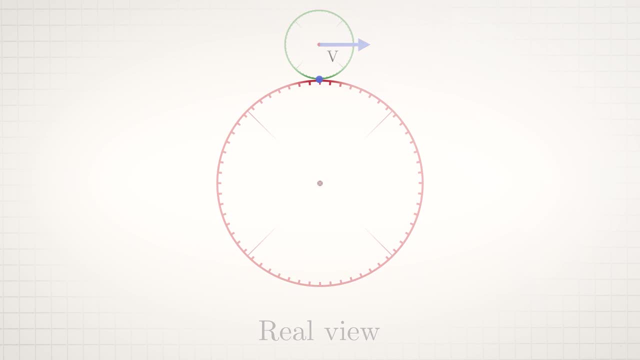 So in your movie it looks like the center doesn't move. In the real world the center is going around the circle. Let's say it's going at some speed V. What's the velocity of this point? It's zero, And that's because it's rolling without slipping. 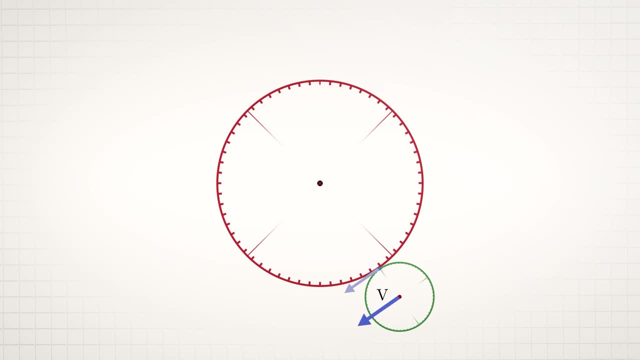 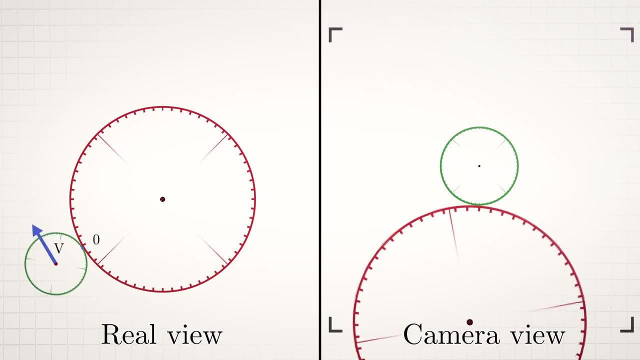 If it had any component in that direction, That's what slipping would be. I mean, this is something I think they should have spelled out in the problem. but when you change your frame of reference, the relative velocities don't change. In the movie, the center always has velocity zero. 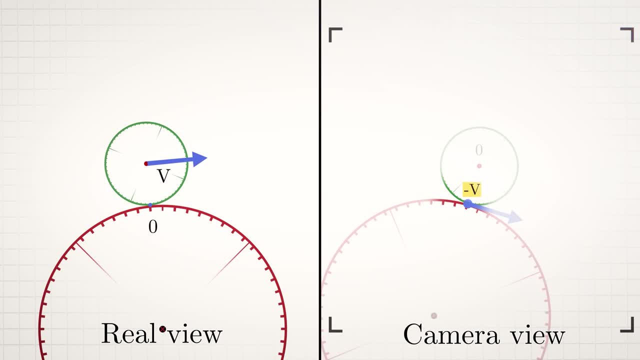 So this point would have to have velocity negative V. So that means the speed that this is turning is the same as the speed the center is moving. So if they always have the same speed, they have to go the same total distance. The total distance. 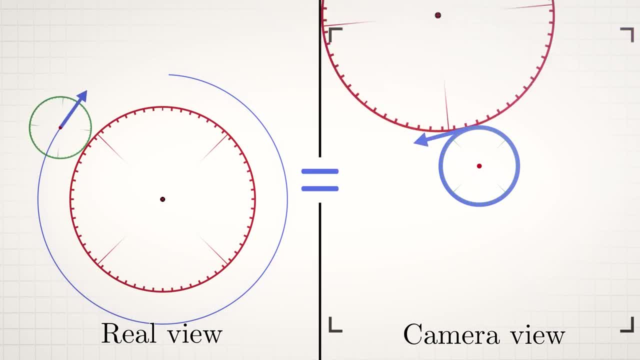 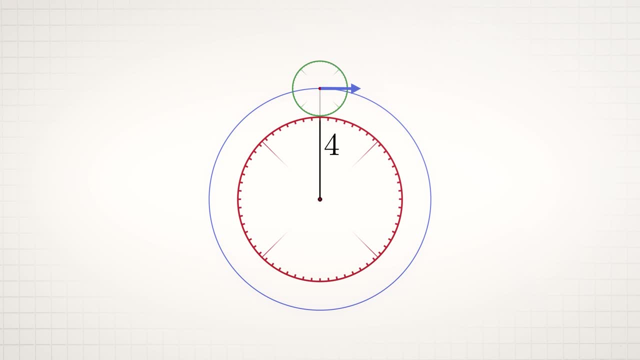 This turns, It's going to be the same as the total distance the center moves. In this problem, the center of the small circle goes around a circle of radius four, So the total distance that the center moves is eight pi. What's the total amount that the small circle rotates? 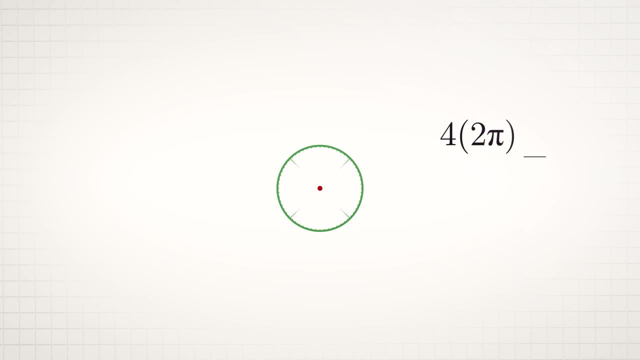 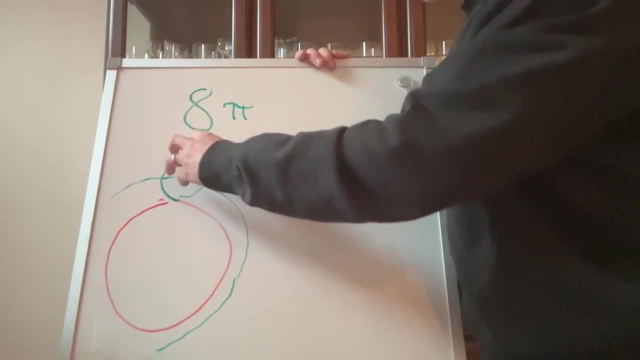 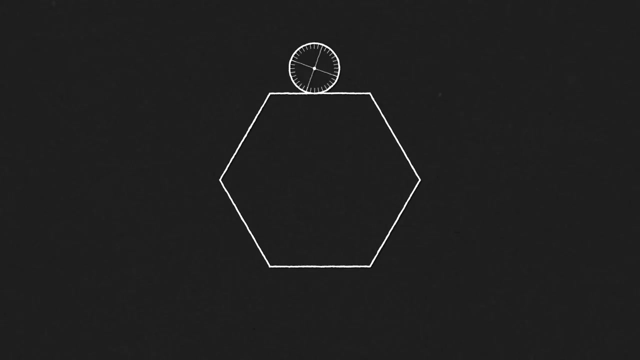 It rotates four times and the circumference is two pi. It's the same number. If it rolls without slipping, the total distance the center travels is the same as the total amount it turns, And this is always true. Take a circle rolling without slipping on any surface, from a polygon to a blob on. 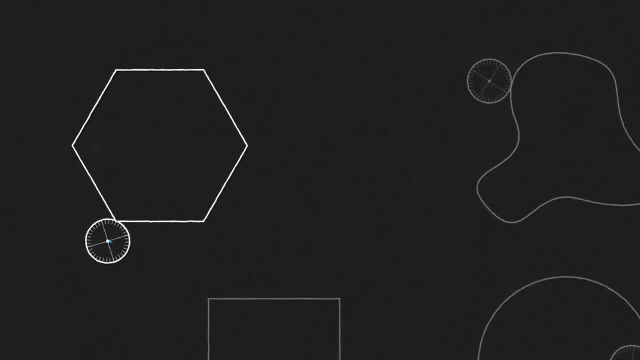 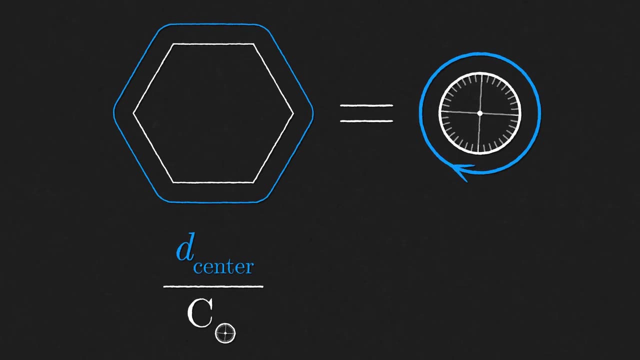 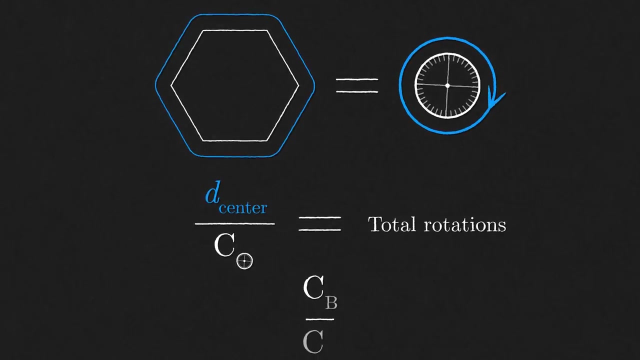 the outside or the inside, The distance traveled by the center of the circle is equal to the amount the circle has rotated. So just find this distance and divide it by the circle's circumference to get how many rotations it's made. This is an even more general solution than our answer to the coin paradox, where we just 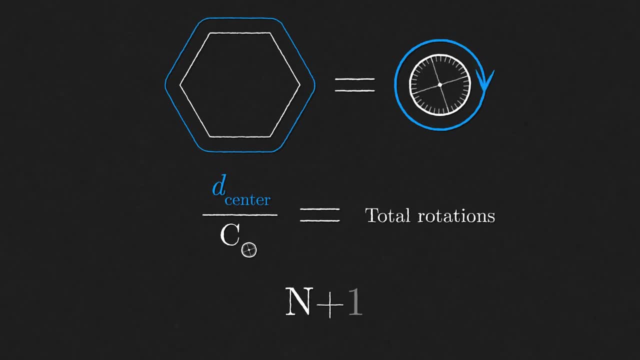 took our expected answer, which we'll call n, and added one pi, And that's it. Thanks for watching. If you enjoyed this video, make sure to hit the like button and subscribe to our channel if you want to see more videos like this one. 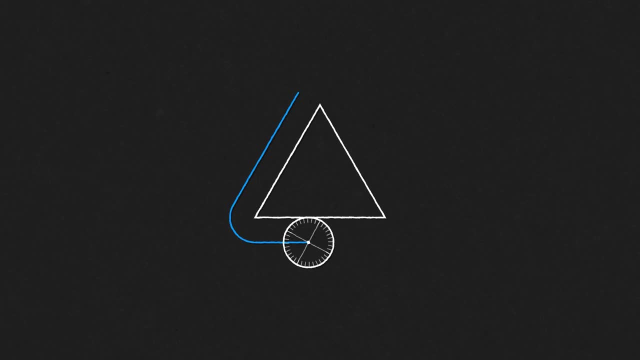 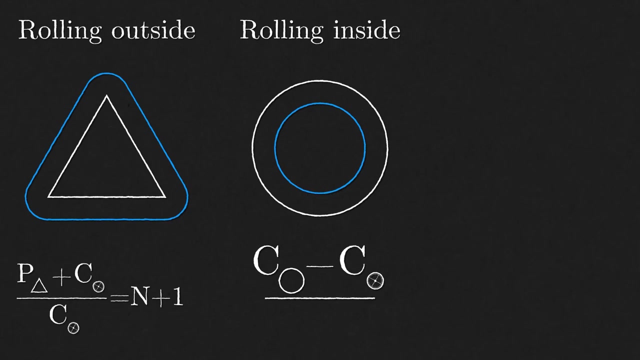 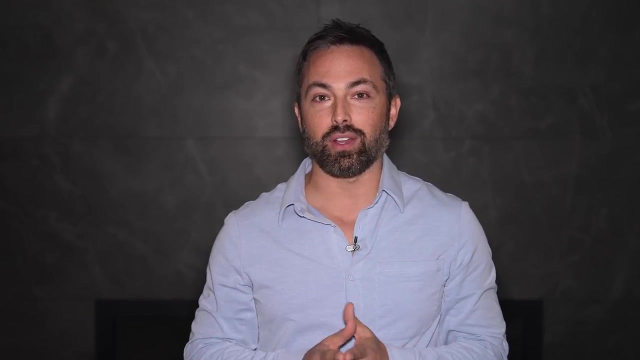 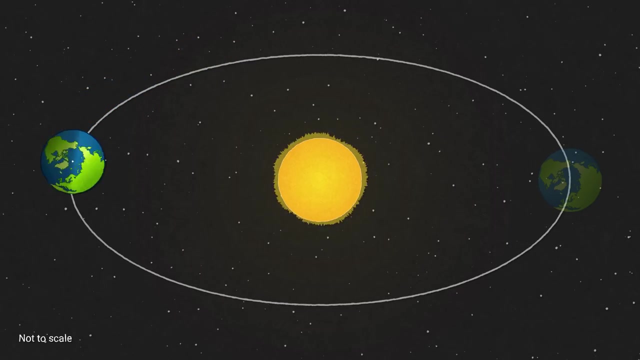 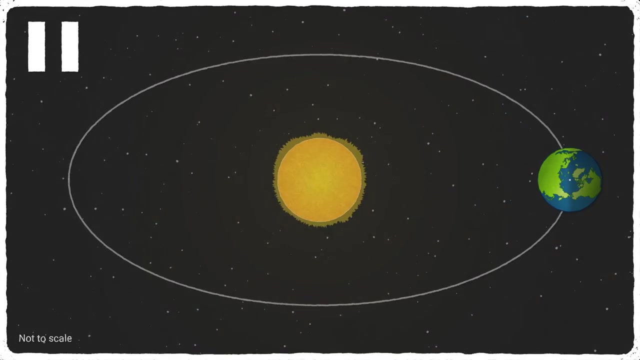 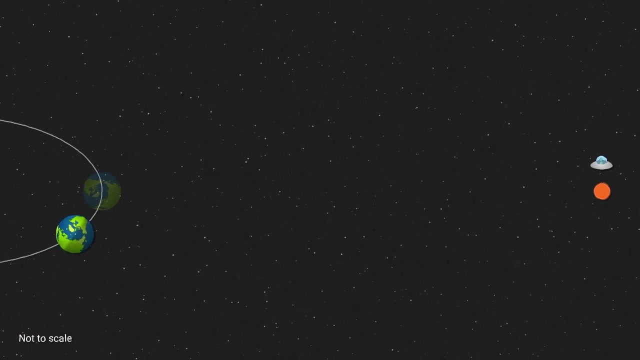 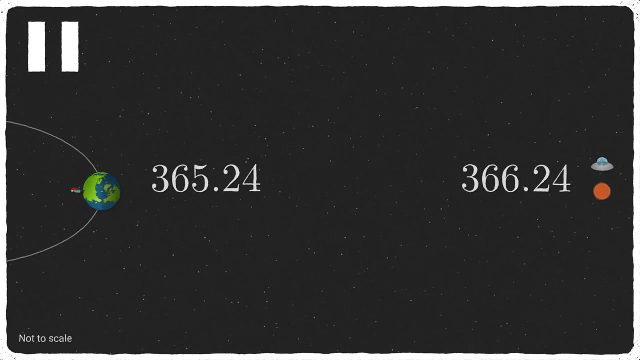 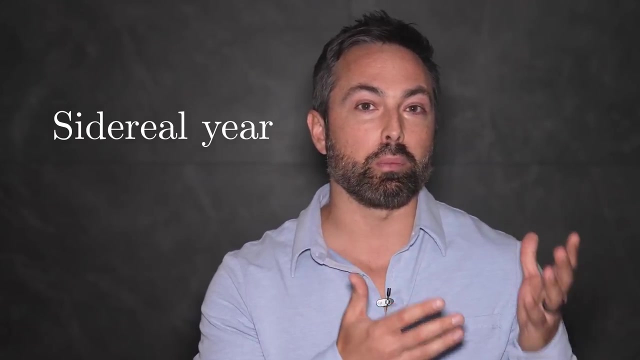 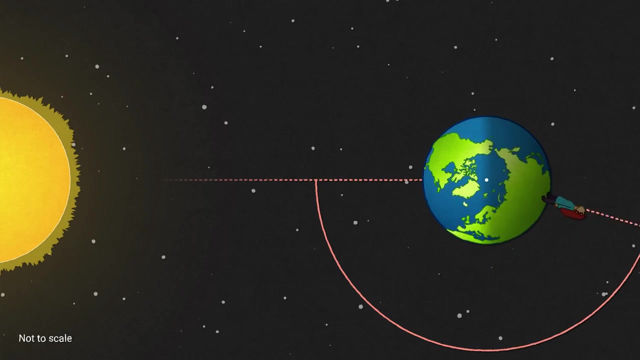 We'll see you in the next video. Bye, Bye. This is called a sidereal year, sidereal meaning with respect to the stars where an external observer would be. But what happens to that one extra day? A normal solar day is the time it takes the sun to be directly above you again on earth. 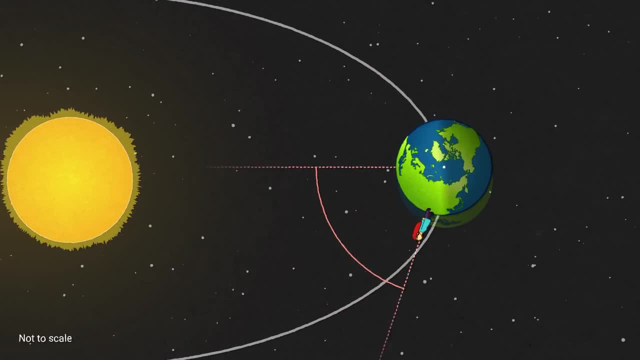 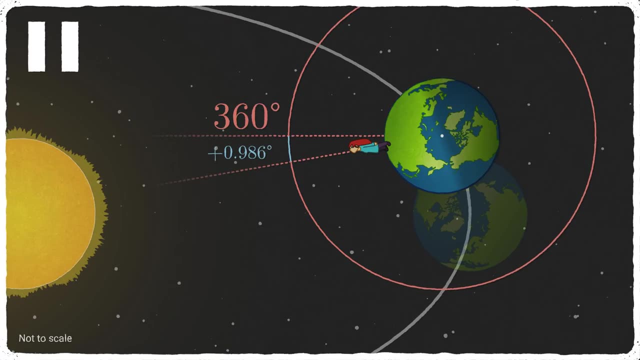 But the earth isn't just rotating, it's orbiting the sun at the same time. So in a 24 hour solar day, Earth actually has to rotate more than 360 degrees in order to bring the sun directly overhead again. But Earth is not the only solar day. 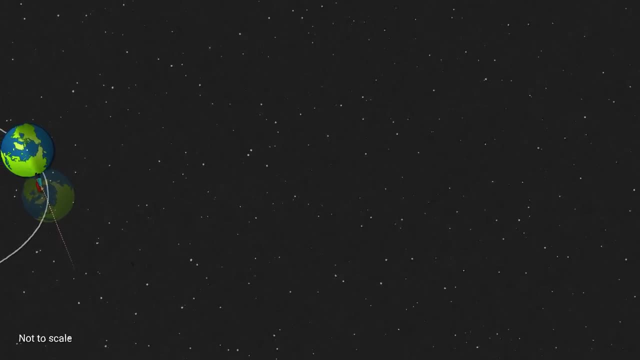 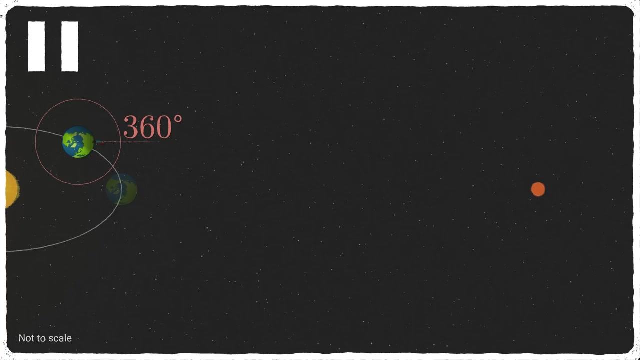 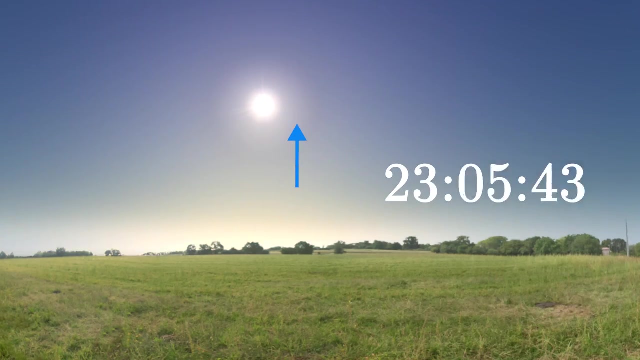 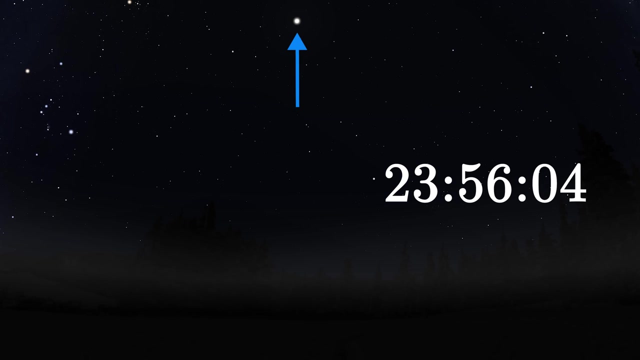 Earth's orbit is negligible to distant stars. To see a star directly overhead again, Earth just needs to rotate exactly 360 degrees. So while it takes the Sun exactly 24 hours to be directly above you again, a star at night takes only 23 hours, 56 minutes and 4 seconds to be above you again. 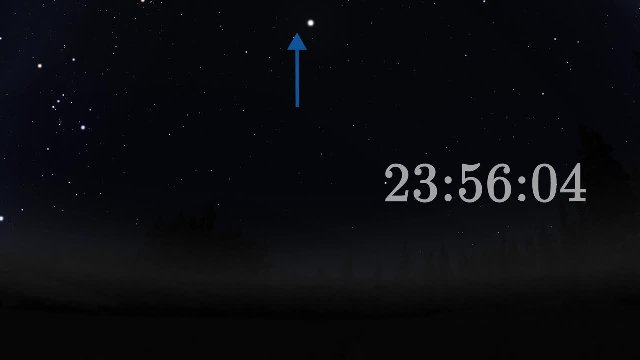 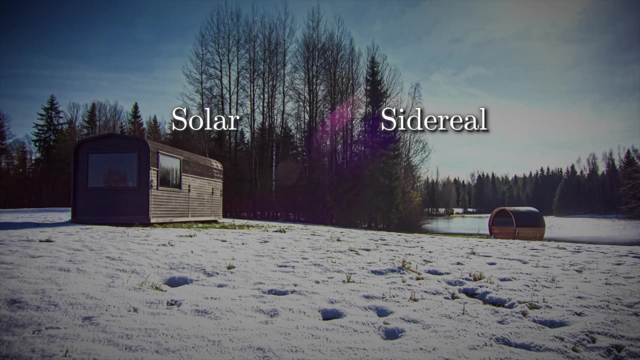 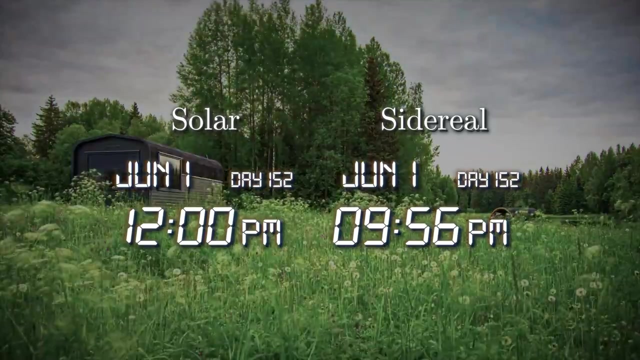 That's a sidereal day. This explains where the extra day goes in the sidereal year. If we start a solar day and a sidereal day at the same time, we'd see them slowly diverge throughout the year. After 6 months, the sidereal day would be 12 hours ahead of the solar day, meaning that noon would be midnight, and it would keep moving up until it's finally one full day ahead of the solar day, at which point a new year and orbit begins 360.. 365.24 days that are each 24 hours long are equal to 366.24 days that are each 23 hours. 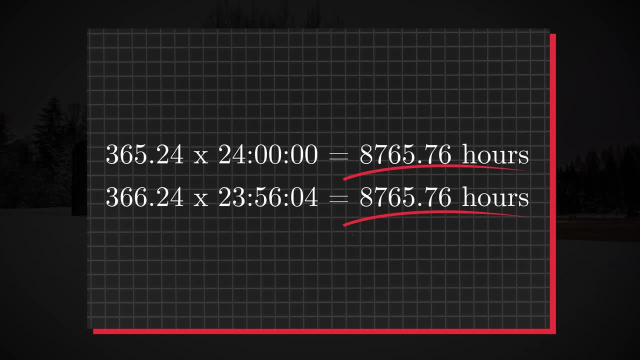 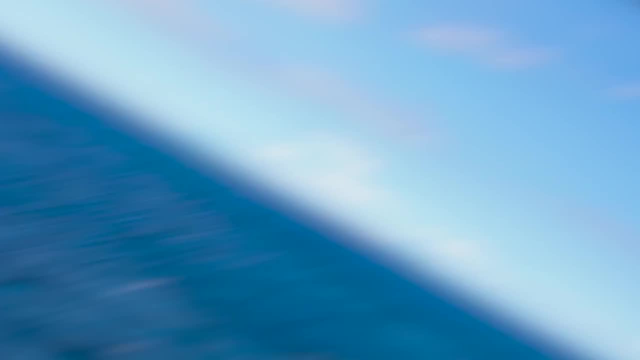 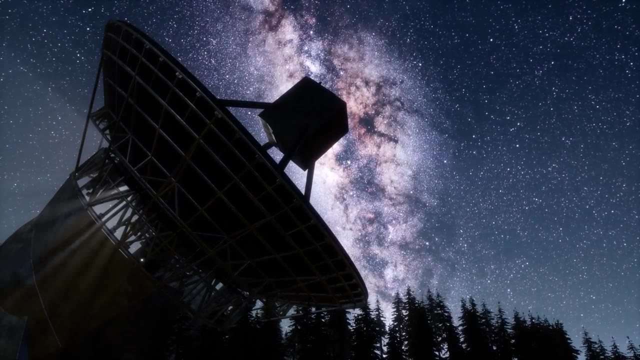 56 minutes and 4 seconds long. So it makes no sense to use sidereal time on Earth, because 6 months down the line, day and night would be completely swapped. But equally it's useless to use solar time while tracking objects in space, because the 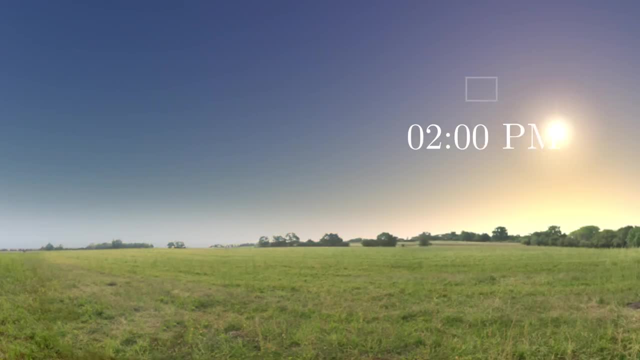 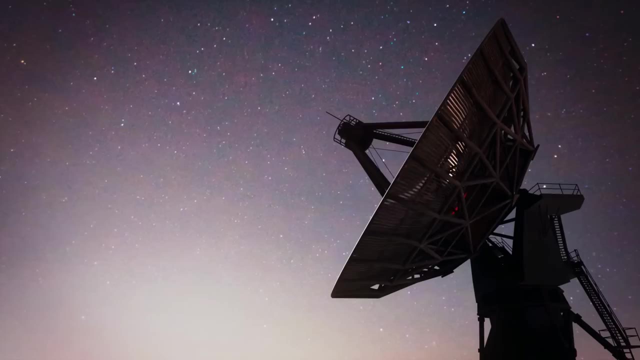 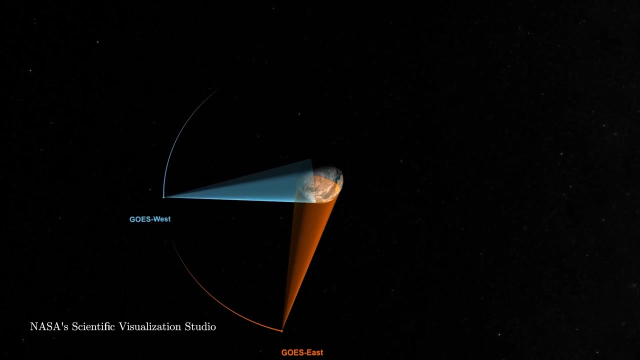 region you're observing would shift. So instead, astronomers use sidereal time for their telescopes to ensure that they're looking at the same region of space each night, And all geostationary satellites, like those used for communication or navigation, use. 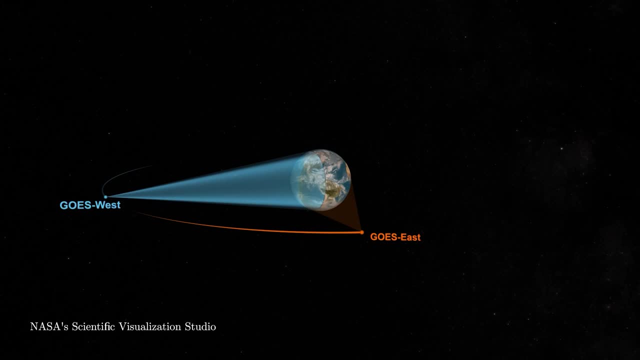 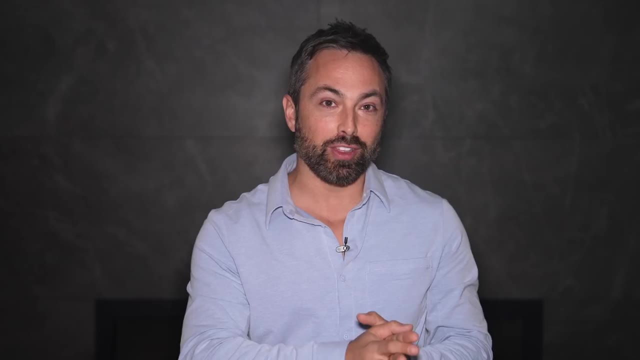 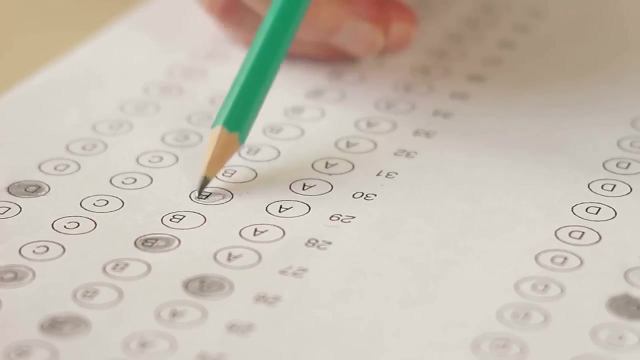 sidereal time to keep their orbits locked with the Earth's rotation. So the coin paradox actually explains the difference between how we track time on Earth and how we track time in the universe. The re-scoring of the 1982 SAT wasn't all good news. 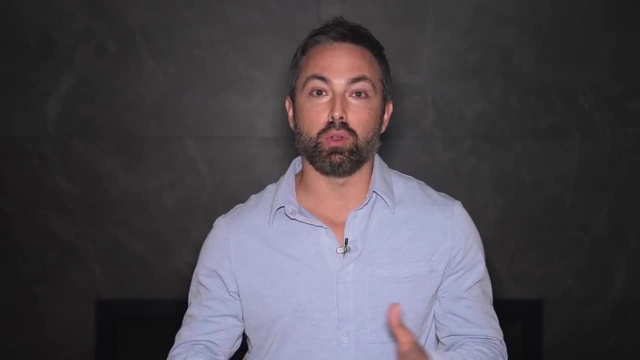 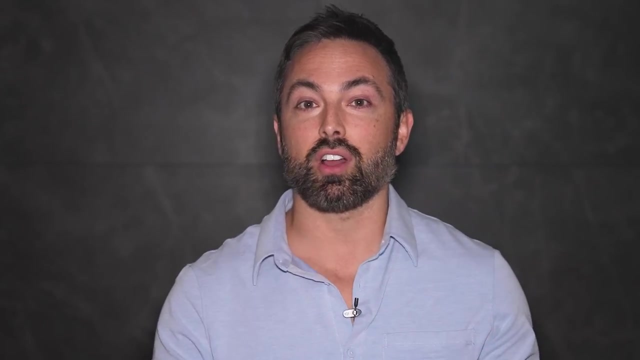 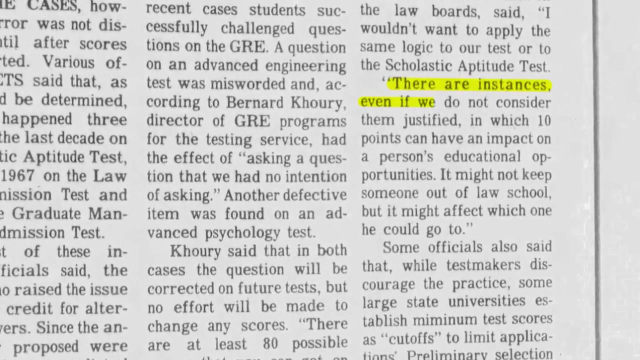 With Question 17, scrapped students' scores were scaled without it, moving their final result up or down by 10 points out of 800.. While that doesn't seem like much, some universities and scholarships use strict minimum test score cut-offs And, as one admissions expert put it, there are instances even if we do not consider. 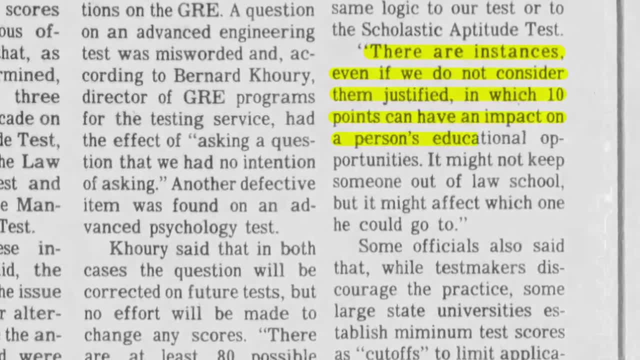 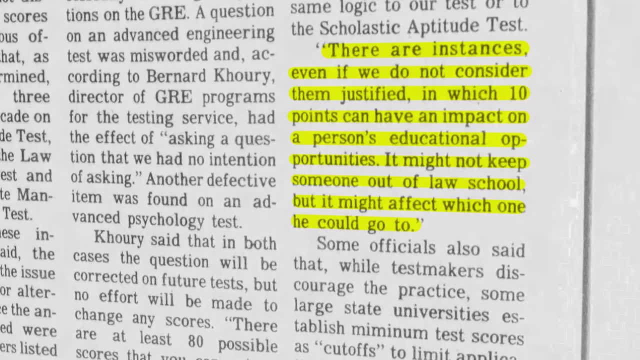 them justified, in which 10 points can have an impact on a person's life. That's what we're looking for. It might not keep someone out of law school, but it might affect which one he could go to. This mistake didn't only cost points off the exam, according to the testing service. 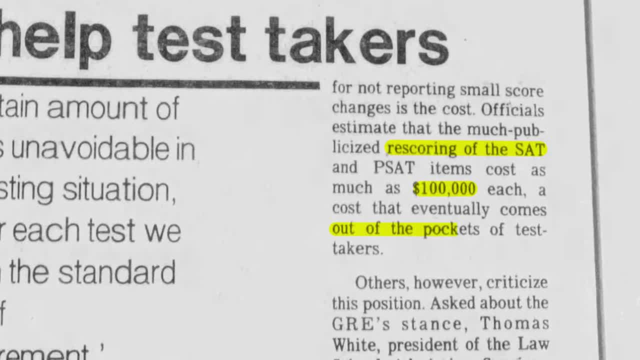 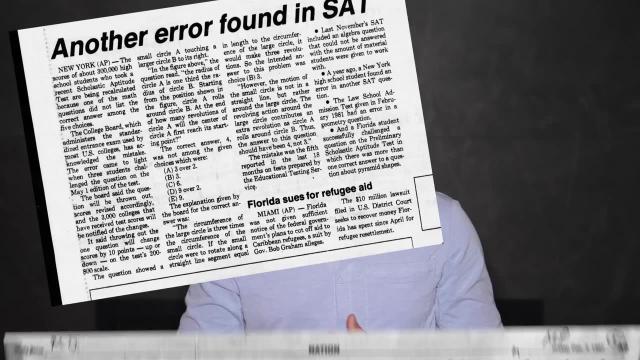 Rescoring would cost them over $100,000, money that came out of the pockets of test takers. The Question 17 circle problem was far from the last error on the SAT, But errors are likely the least of their concerns these days. 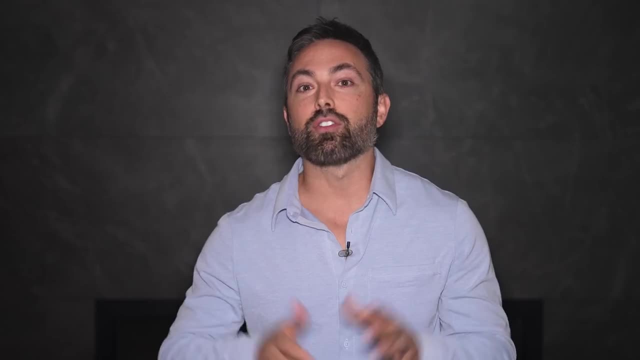 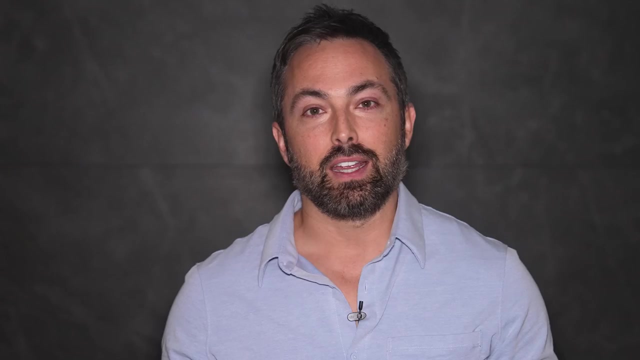 I mean, the SAT is slowly becoming a thing of the past. After COVID-19,, nearly 80% of undergraduate colleges in the US no longer require any standardized testing. And that 1982 exam? well, it didn't turn out too badly for some. 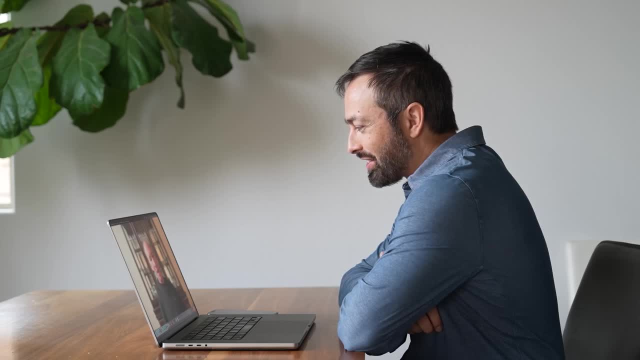 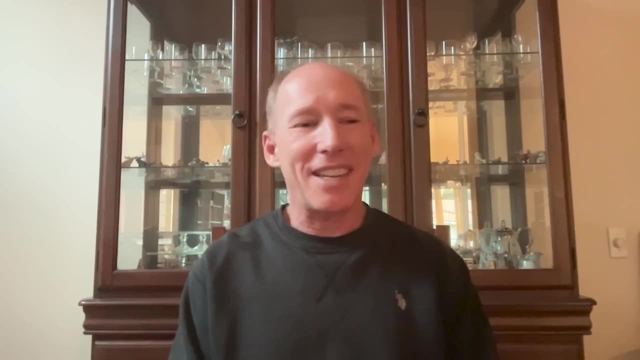 How did you do on your math SAT, if I can ask? I got an 800.. Even before that it was clear I was going to go into math. I did math competitions. I really liked math. Do you end up writing any math questions? 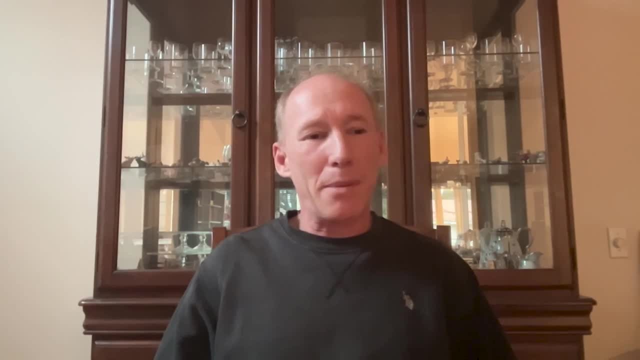 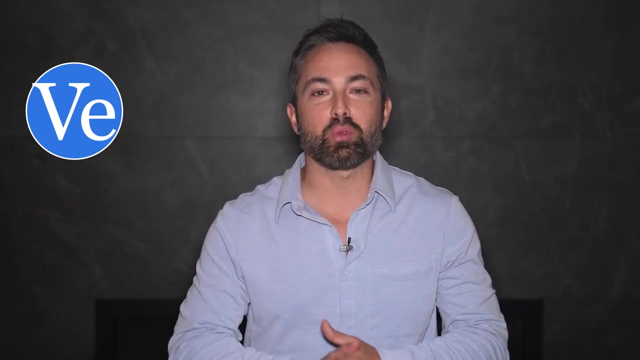 Yeah, Do you write any math questions these days? A while back I wrote problems for a math competition And were you careful with how you wrote them, The wording? I hope so I tried. Today's deep dive on one SAT question proves there's no substitute for hands-on. 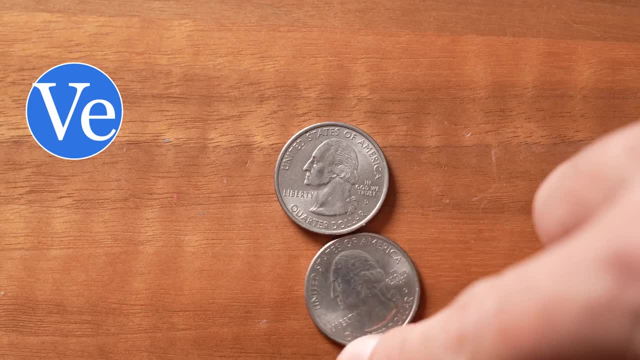 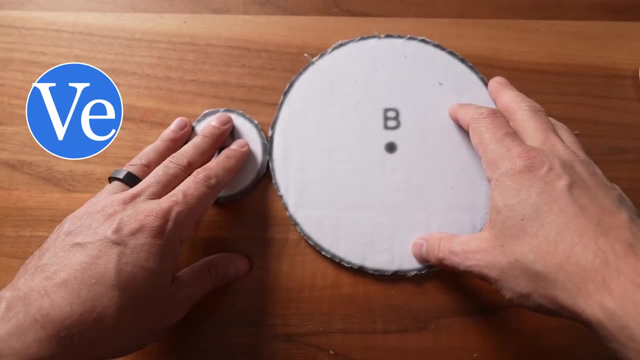 exploration to understand and appreciate the everyday phenomena of our world. But you don't have to observe Earth from space or make cardboard cutouts to get hands-on with math, science and cutting edge. In fact, you can do it from anywhere right now with this video's sponsor, Brilliant. 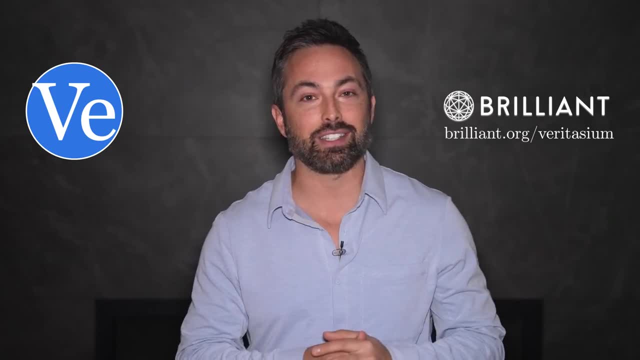 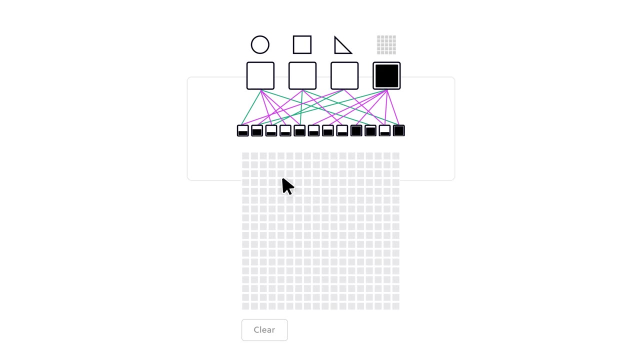 And you can get started for free. Just go to brilliantorg. slash veritasium. Brilliant will make you a better thinker and problem solver in everything from science to math, data programming, technology- you name it. Just set your goal and Brilliant will design a path to get you there. 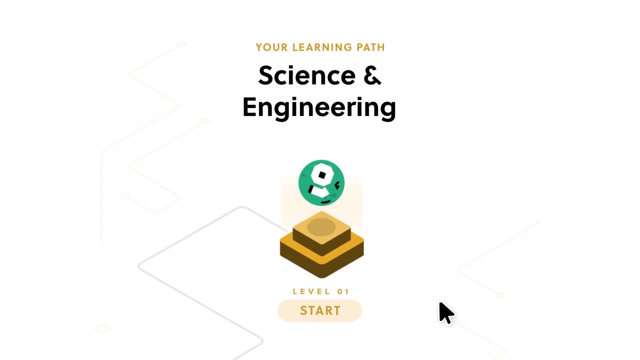 If you liked today's video, I highly recommend you check out one of my favorite courses on Brilliant, which is scientific thinking. Scientific thinking takes you on an interactive tour of our physical world. You'll engage with key scientific principles and theories from simple machines like gears. 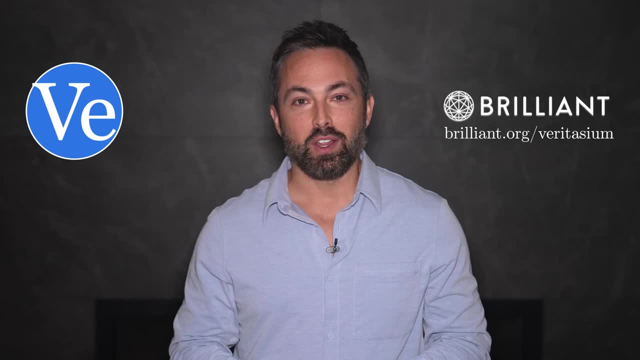 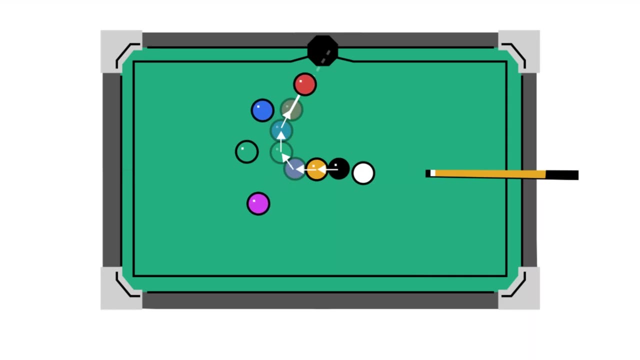 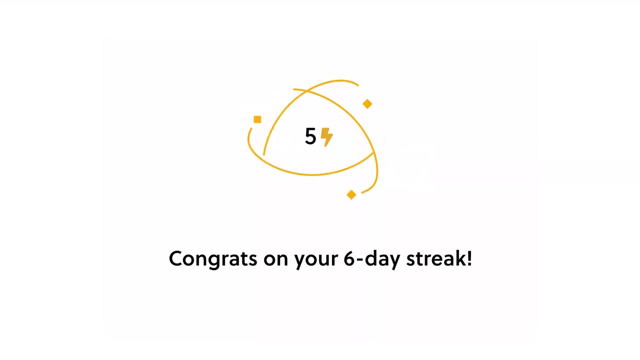 and pulleys to Einstein's special theory of relativity. Whether you're comparing circuits to understand voltage and current, playing snooker to learn the rules of collisions, or even planning your itinerary for an intergalactic music festival on a space-time diagram, you will learn by doing and foster a deep understanding.